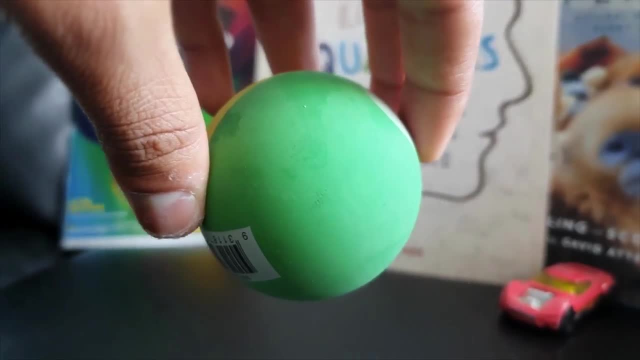 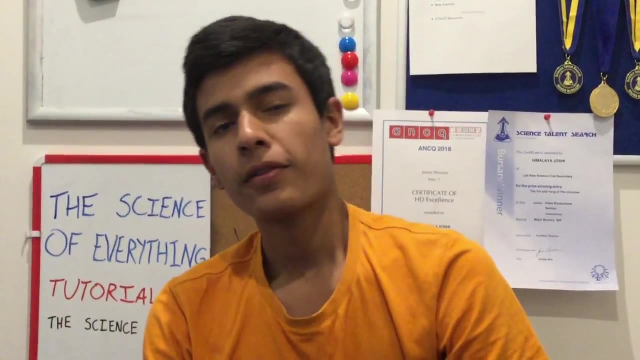 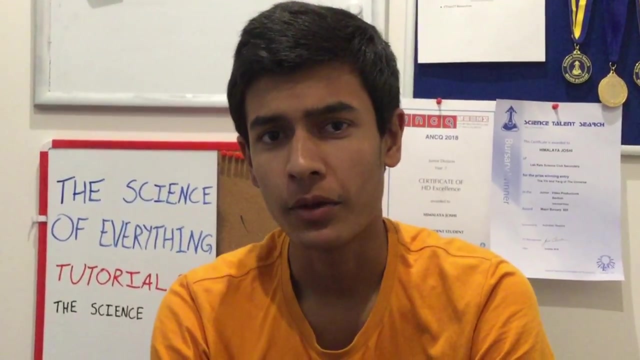 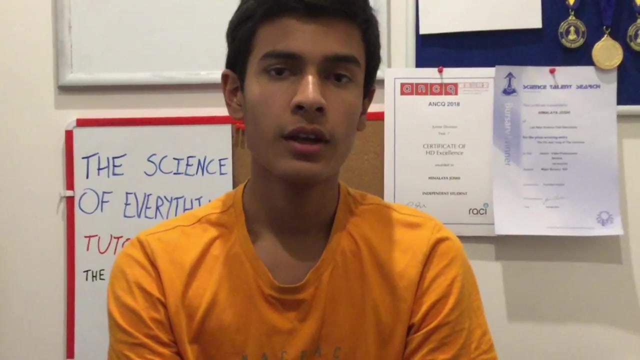 know. Now that I've announced the three important things I was going to announce, let's get straight into this video. Think back to year 7 and 8, high school physics. Let me guess you probably learnt about the basics behind forces. You learnt about gravity, friction and the normal force. Now these 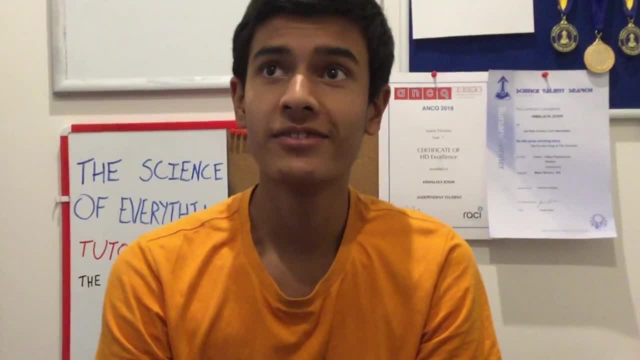 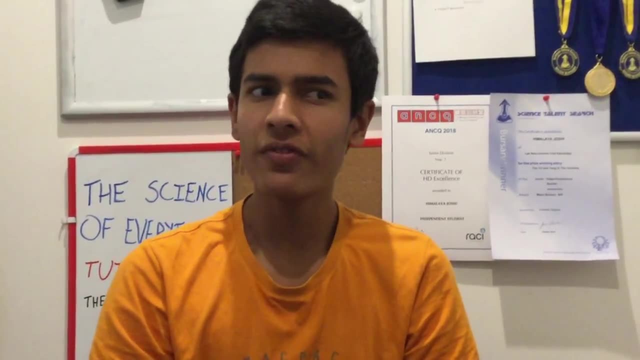 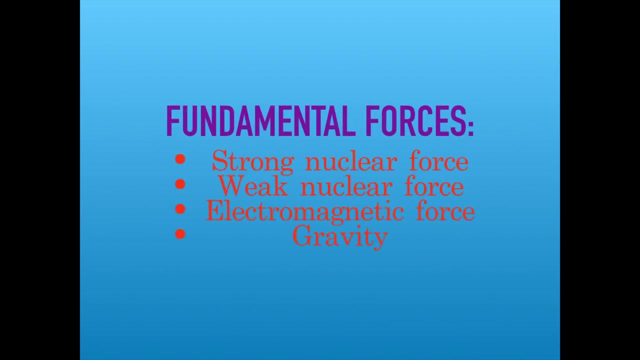 forces do apply to the macroscopic world, that is, the big world we live in, But down at the quantum scale we talk about the fundamental forces, not these classical ones, because they don't work. The four fundamental forces of nature are the strong nuclear force, the weak nuclear. 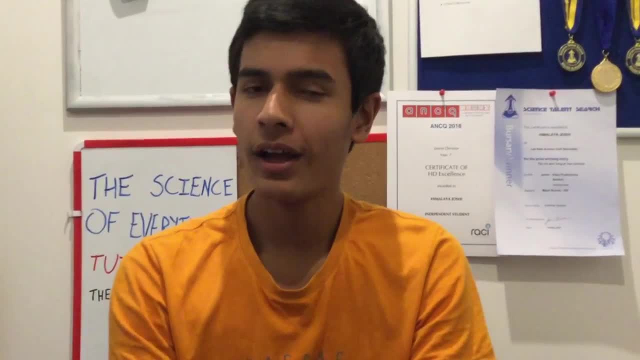 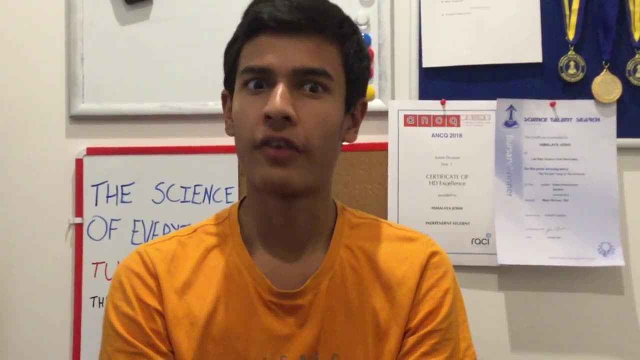 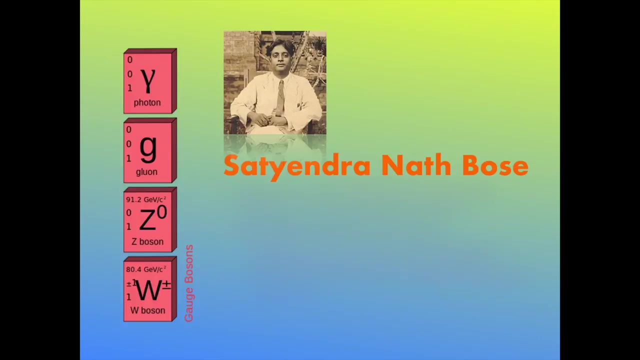 force- the electromagnetic force and gravity- And in this tutorial, we're shortly going to be learning about the particles that help carry these fundamental forces. These particles are called bosons, and they're named after the Indian particle physicist, Satyendra Nath Bose. Bosons are the particles by which the influence of fundamental forces 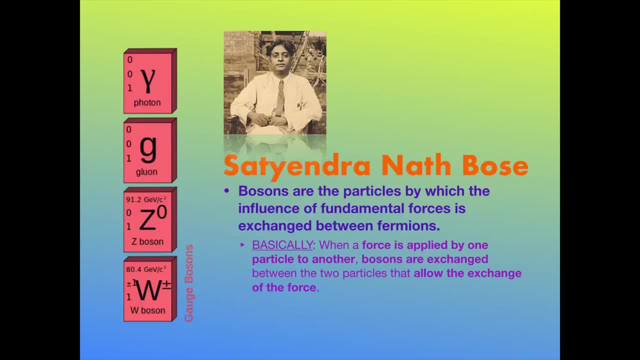 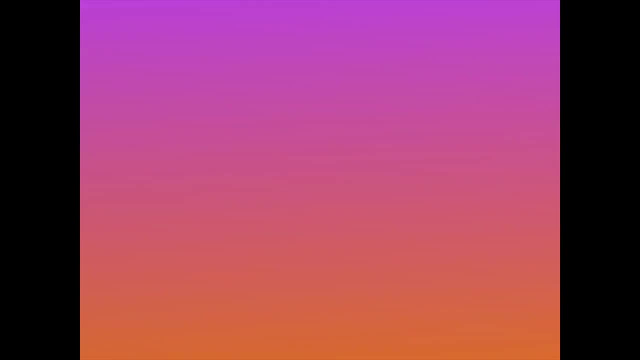 is exchanged between fermions. Basically, when a force is applied by one particle to another particle, bosons are exchanged between the two particles that allow the exchange of that particular force. Now, the Higgs boson is one boson that we won't be talking about in this tutorial, Because 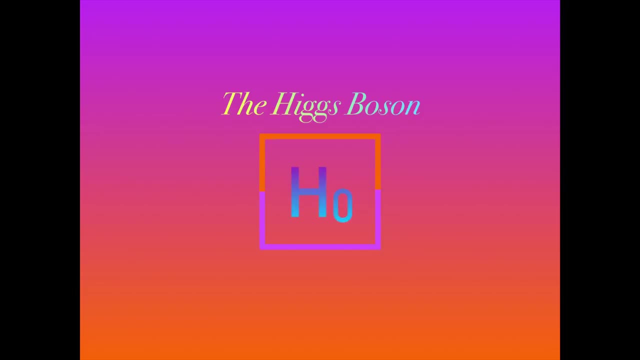 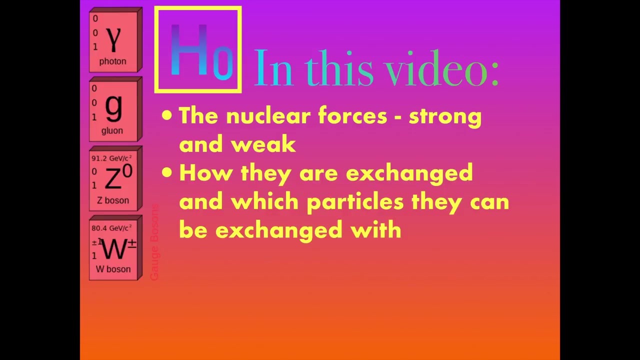 this boson is so special that it deserves a video on its own, And that video is not this video. That is for another tutorial. In this video, we're going to be learning about the strong and weak nuclear forces that exist within a nucleus and how they're exchanged between particles, and which particles they 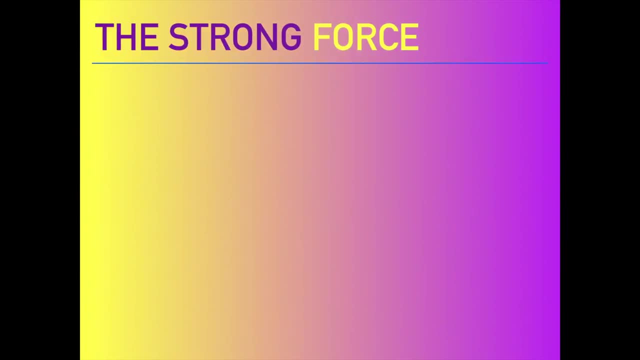 can be exchanged with. Let's discuss the strong force first. The strong force is the strongest of all fundamental forces of nature. Moreover, it can be felt by all quarks and hadrons. Hadrons are basically any particles that are made up of a multiple number of quarks. 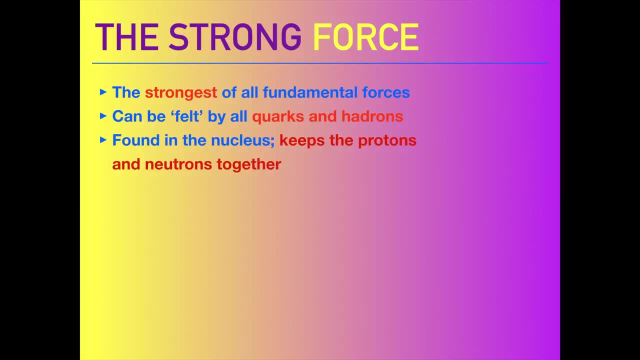 And the strong nuclear force exists in the nucleus And it keeps the protons and neutrons together. It's called the strong force because it's stronger than the electromagnetic force in the nucleus Because, remember, there are many protons in a nucleus and protons are positively. 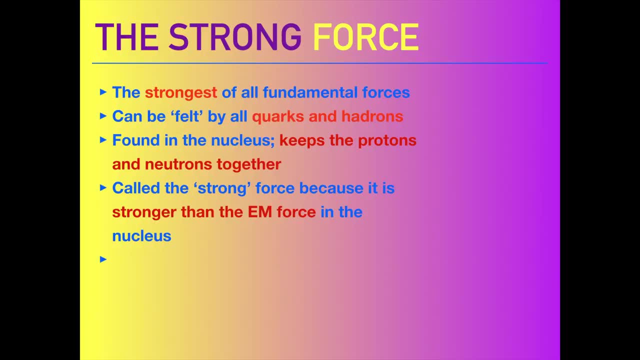 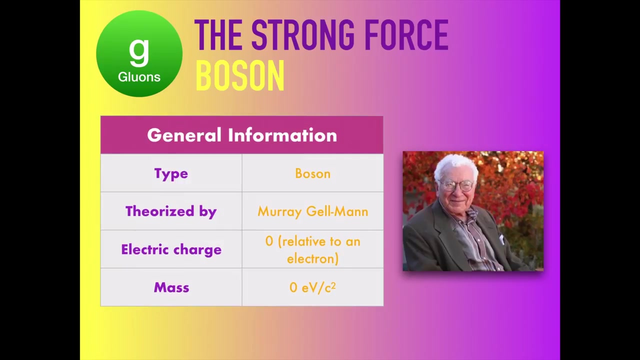 charged, which means they should be repelling each other. But something keeps them together, And that is the strong nuclear force. And they're exchanged by gluons and mesons. Let's talk about the gluon. The gluon is the boson that allows the exchange of the strong nuclear force. It was theorised. 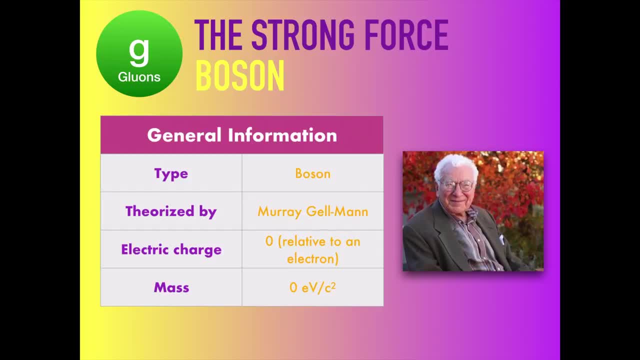 by Murray Gell-Mann and has an electric charge of zero relative to an electron and has a mass of zero as well. It's called a gluon because, literally, it glues things together, It glues things together. It's called a gluon because, literally, it glues things together, It glues things together. It's called a gluon because literally it glues things together. It glues things together And it's called a gluon because literally it glues things together. It can glues protons and neutrons together to form a nucleus. 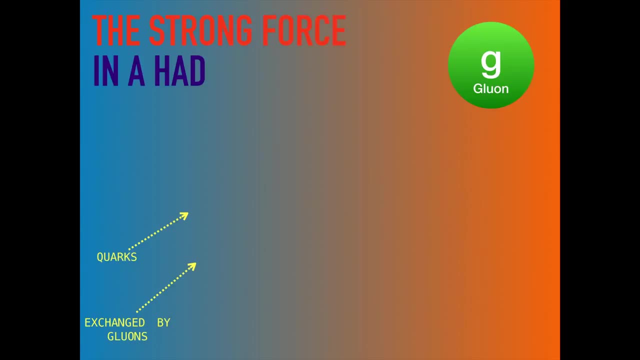 Let's talk about the existence of the strong force in a hadron, In particular the proton. That's our pretty diagram of a proton. So, as you can see here, between the two up quarks and the one down quark, the strong. 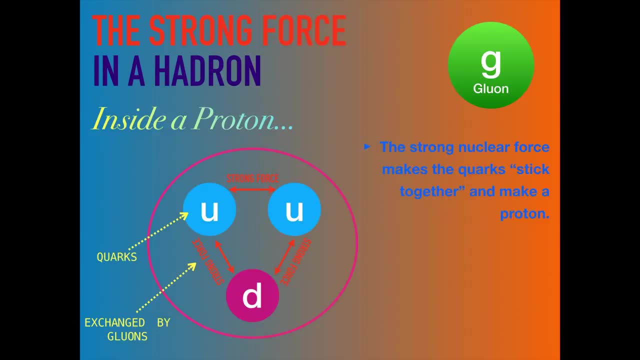 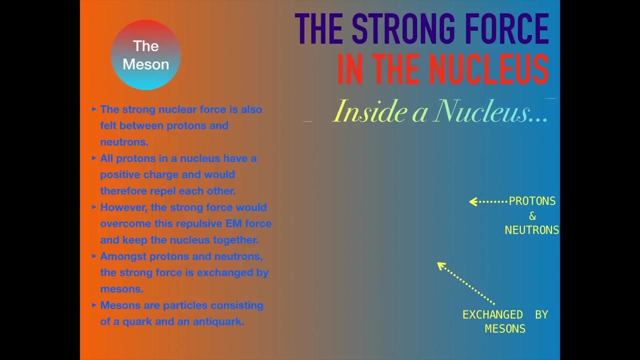 force is being exchanged by gluons. The strong nuclear force makes the quarks stick together and make the proton. The same thing happens occurs in any hadron, including a neutron or a pion. The strong force not only exists inside individual hadrons, but it also exists inside a nucleus. 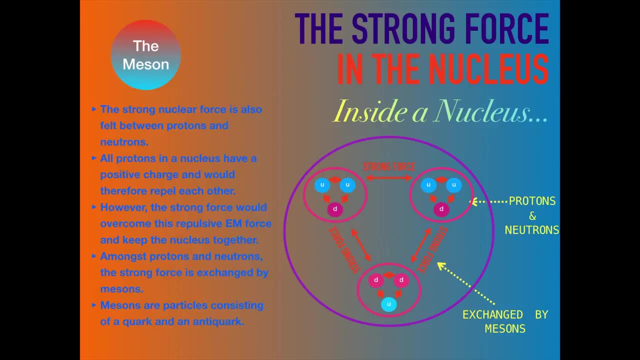 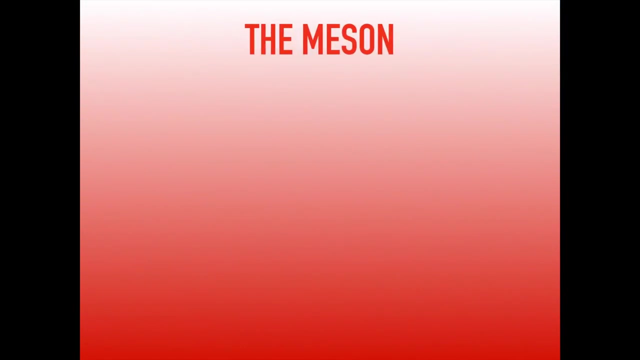 As we can see here, the strong forces exchange between protons and neutrons not by gluons but by mesons. All the protons in a nucleus have a positive charge, but they don't repel each other because they're kept together by the strong force. 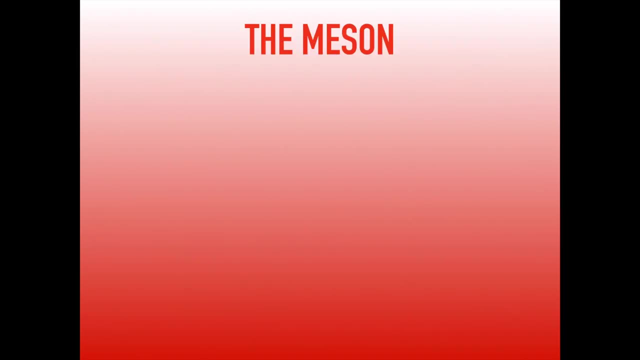 I've mentioned the word meson quite a few times now. What do I really mean by it? Well, a meson is basically any type of particle consisting of a quark and an antiquark. The general structure of a meson is any of the six types of quarks and any of the six. 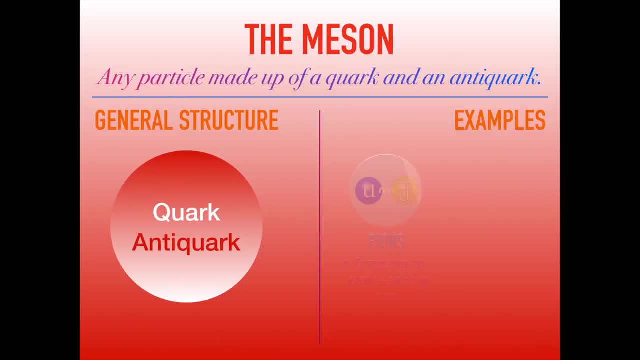 types of antiquarks. Two examples of mesons are pions consisting of one up quark and one anti-down quark, and kaons consisting of one up quark and one anti-strange quark. If you don't know what a meson is, you'll know in a minute. 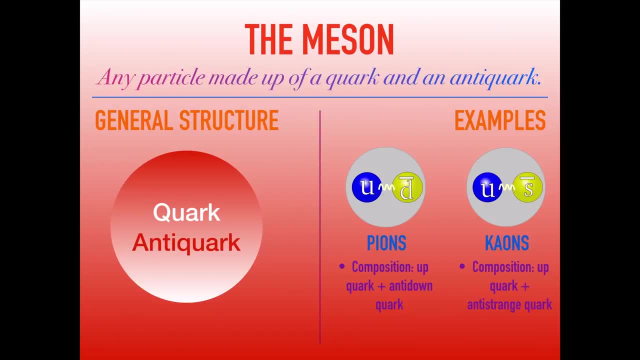 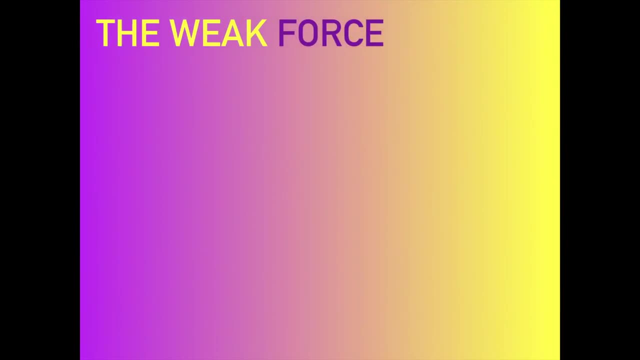 If you don't know what quarks, leptons or fermions are, just watch my first tutorial of the science of everything, and that should clarify everything for you. Okay, now that we've racked our brains with information about the strong force, let's. 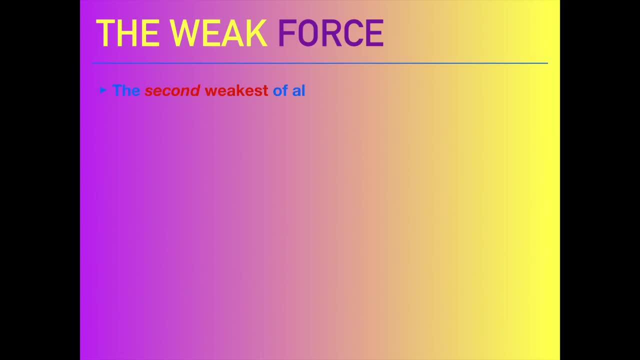 learn about the weaker side of things: the weak force. The weak force is the second weakest of all fundamental forces. If you want to know what the weakest of all forces is, well, you're going to have to wait until another tutorial. Also, it can be felt by all fermions. 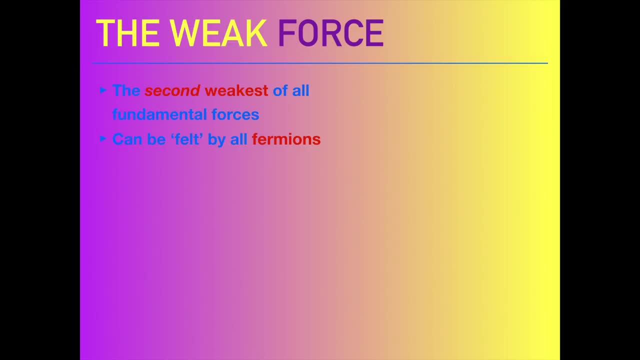 Unlike the strong force, which can only be felt by quarks, The weak force can be felt by both quarks and leptons, And it doesn't make particles stick together like the strong force does. It does well other weird things. 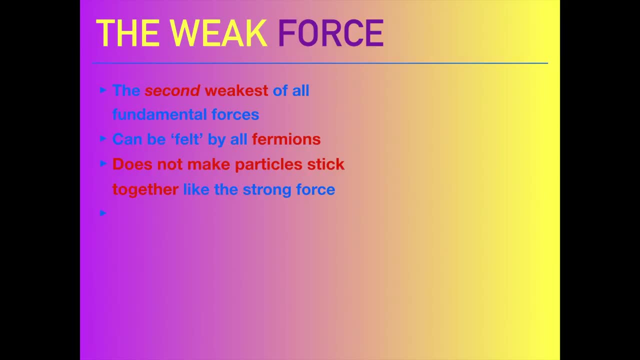 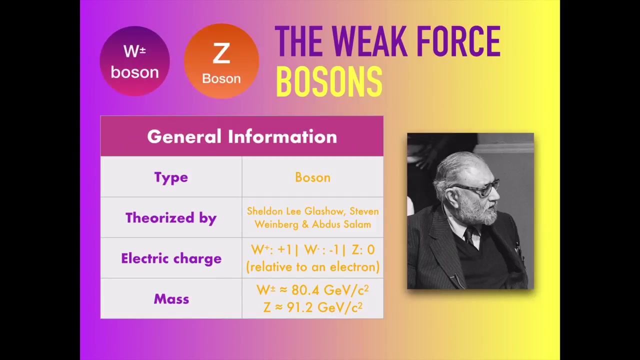 It makes particles change types between each other, It's responsible for bizarre particle changes And it's exchanged by quarks. The weak force can be felt by two different types of bosons: The W bosons and the Z bosons. Let's talk about the weak force bosons: the W and the Z bosons. 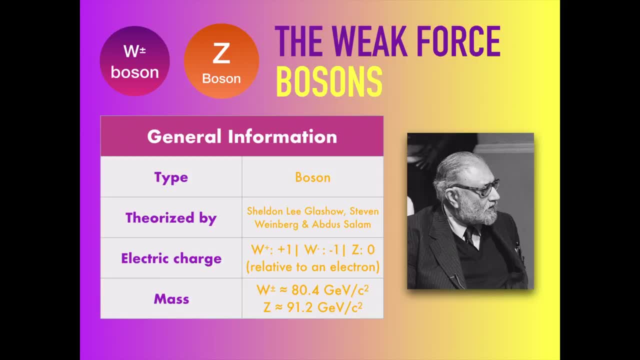 These two particles were theorised by Sheldon Lee Glashow, Steven Weinberg and Abdus Salam. The W plus boson has a charge of positive one, while the W minus boson has a charge of negative one. The Z boson remains neutral. 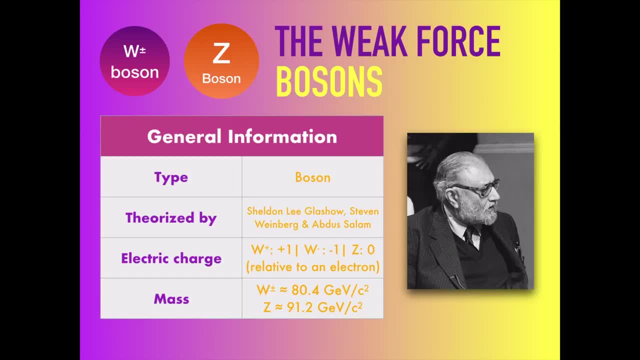 The W plus boson has a charge of positive one, while the W minus boson has a charge of negative one. The Z boson remains neutral. Both bosons have a mass of around 80 gigaelectronvolts per speed of light-squared. 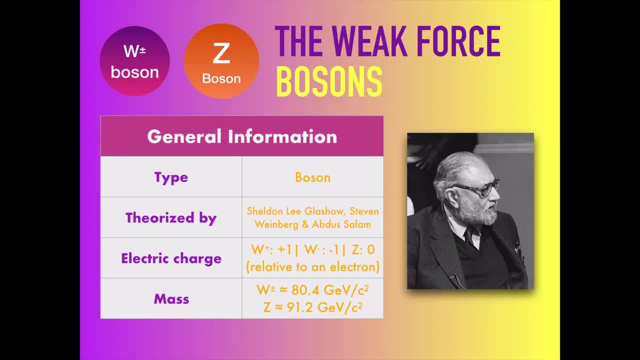 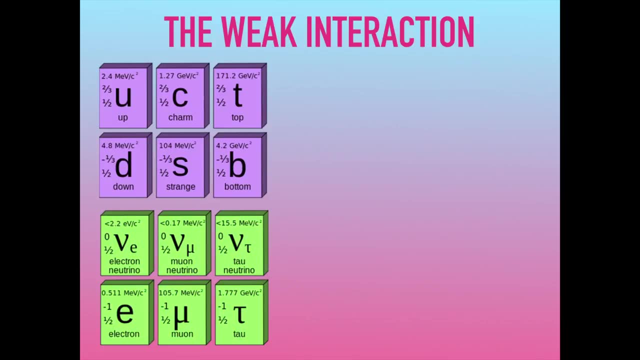 Whereas the mass of a Z boson is around 11 more than that. Remember how I talked about the weak force being responsible for bizarre particle changes? Well, the technical term for those bizarre particle changes is the weak interaction. The weak interaction takes place between the up-type quarks and the down-type quarks, and 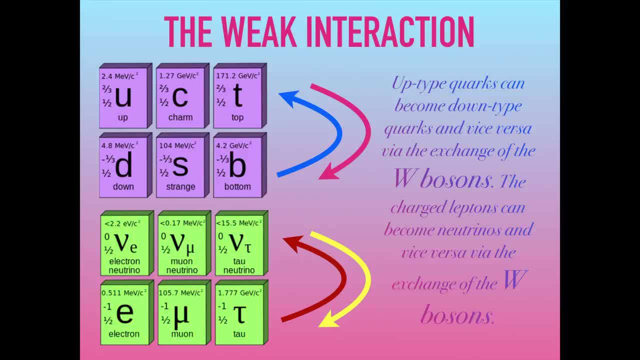 the charged leptons and the nucleus. So these reactions are called физangerous changes because of a physical change within a particle's matrix. Now let's talk about the signs of repulsion. Up-type quarks can transform into down-type quarks and vice versa, and same with the charged